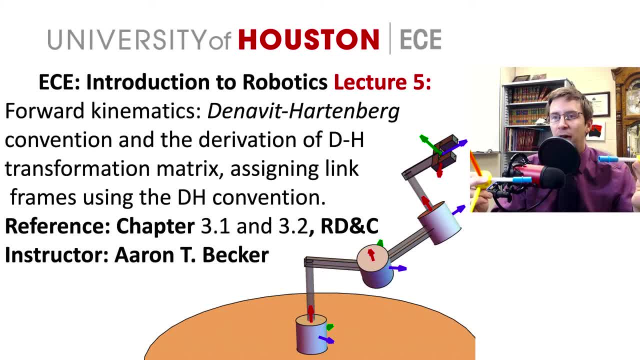 this lecture you'll know how to put all the coordinate frames, like you're on this picture, this three joint RRR robot. This is out of chapters 3.1 and 3.2 of first edition of Robot Dynamics and Control. There's a lot of great resources for this, but my favorite 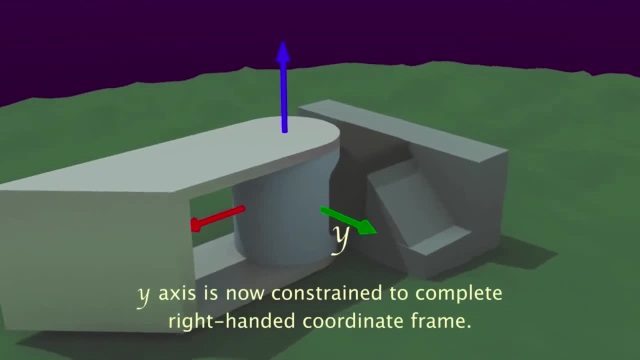 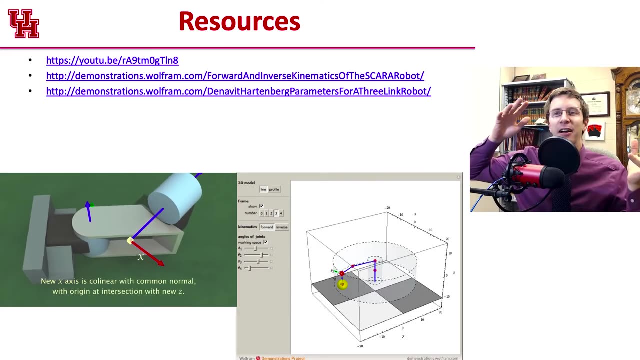 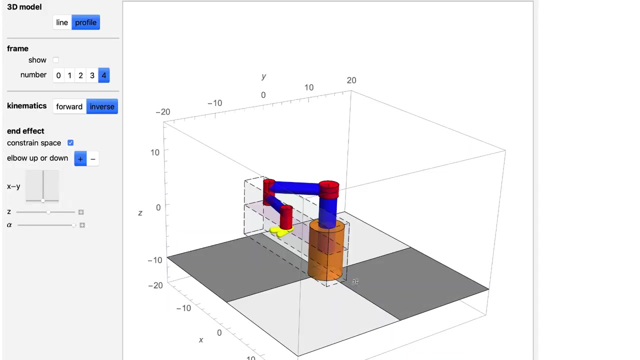 is this YouTube video. It's so important that I watch it a couple times each time I teach the course. I think you should definitely watch it a few times. There's also this nice Mathematica demonstration about the SCAR robot that you can try out. So here's that simulation. If we do our 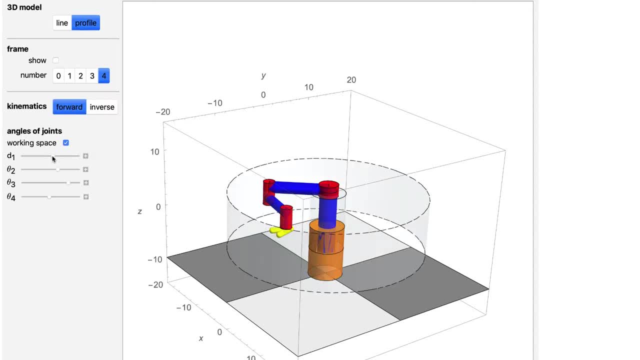 forward kinematics, then we can set the different joints. Our SCAR robot we can translate up and down and we can move our theta one anywhere Around this rotation here and our theta three is rotating over here and we've got a theta four which rotates into factor gripper. Now they have also done their inverse kinematics and they have 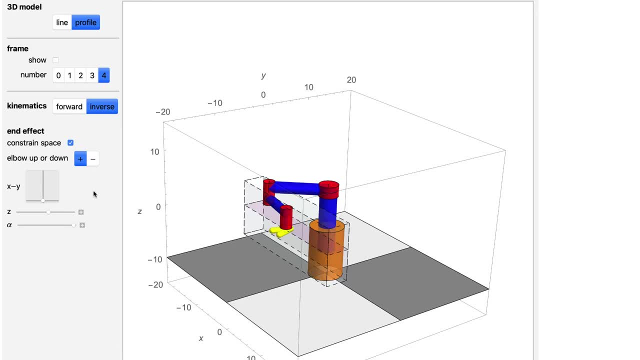 constrained the workspace here so they only have a single solution inside here, So you can move around in your XY workspace and it'll automatically solve out where these joints will be. We're going to learn how to do this in class. You can also pick your Z depth that you're at. 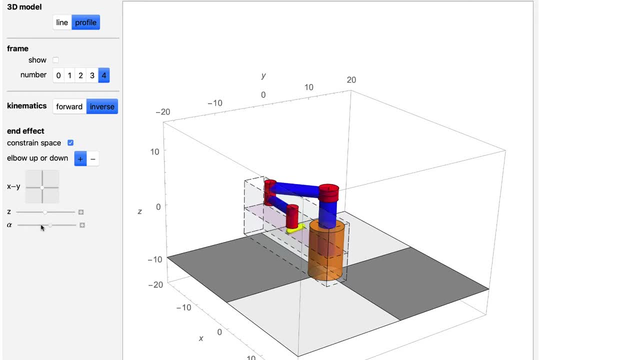 And your alpha value for your final rotation. and then remember there are multiple solutions. So even in this restricted workspace, there is the elbow up and the elbow down solutions. As we move through there, there's going to be two solutions for every point inside this workspace here, But that is this. 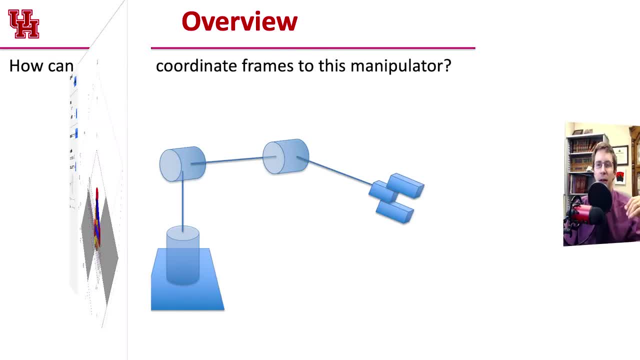 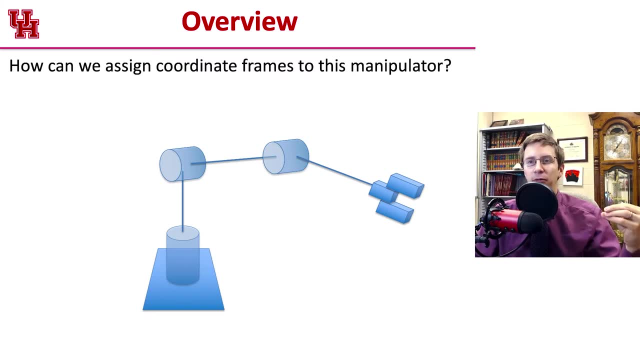 SCARA manipulator. It's a pretty little demo, But again, our big goal is to take some robot which has a number of joints and then assign coordinate frames to it. So we're going to do that here. We're going to assign coordinates to each joint And so at the end of it we're going to be able to go. 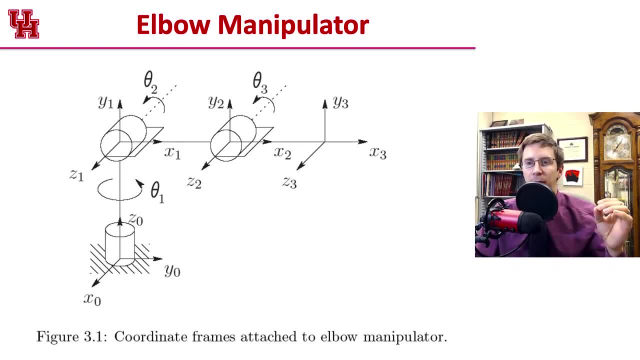 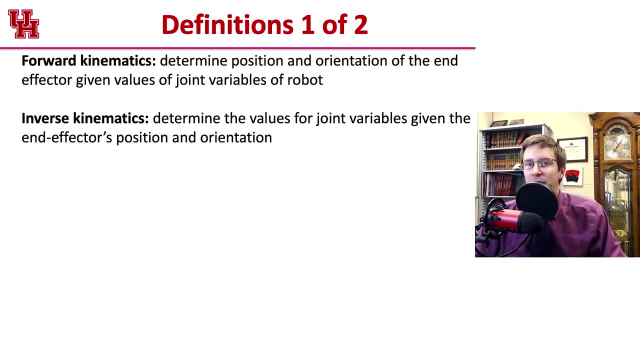 from just a picture of a robot to having the joint frames and the direction of all the movements written on to the image. So it's good to start with some definitions. Remember forward kinematics. we want to know what is the position and the orientation of the end effector. If somebody tells 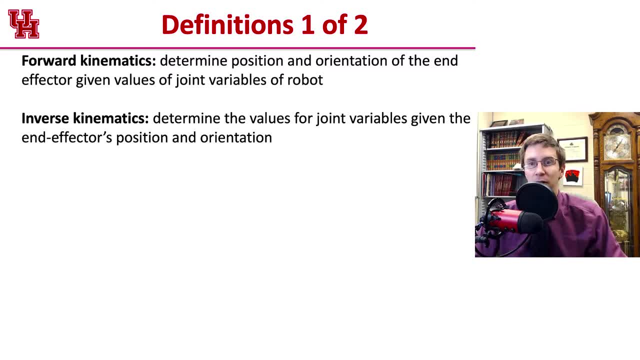 me what all the values are for the joint variables. So those are the angle of rotational joints and the sense of movement of the prismatic joints. Later we're going to talk about inverse kinematics, which is going back the opposite way. So somebody tells me this is where I want the end effector at. 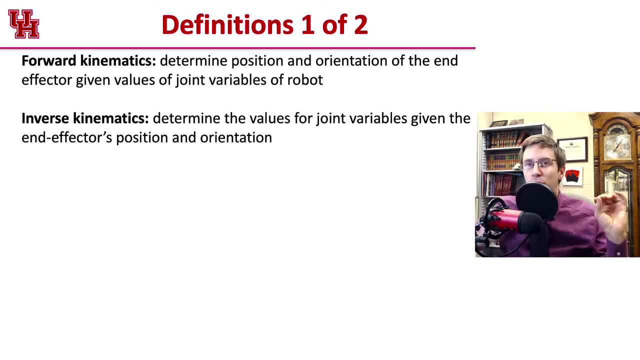 a certain position in orientation. You tell me what should all the joint variables be in order to get there? So we have a rule that each joint is going to be only one degree of freedom. In this class we only have two different joints. The first one is a prismatic joint that can slide back and 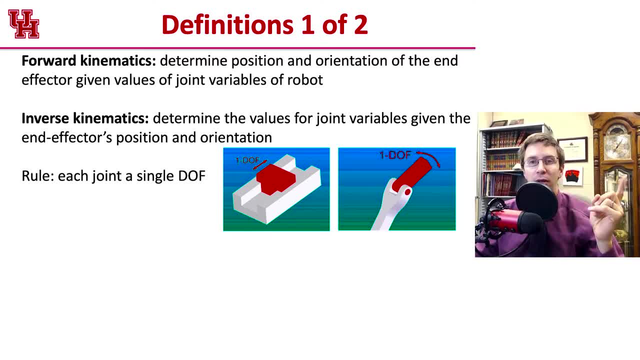 forth. The next one is a rotational joint That can rotate about an axis. Now there also exist joints that have multiple degrees of freedom, such as the two degree of freedom universal joint, or the spherical wrist, which we've already talked about, which has three joints that all meet at the same wrist center point. And so, in this, 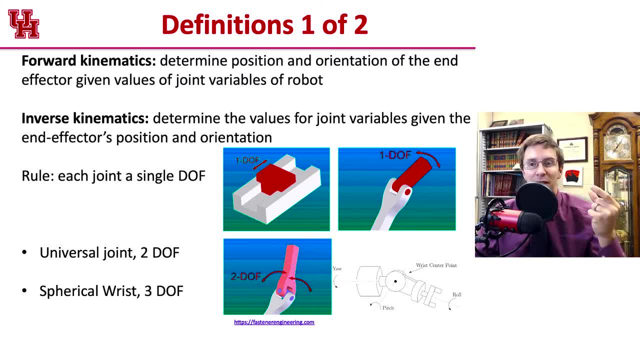 class. whenever we have multiple joints, we're just going to say that there is a zero link length between two successive joints. So we'll just put two joints and we'll have some overlapping frames. So the robot is going to have one more length than the number of joints it has. So we're going to 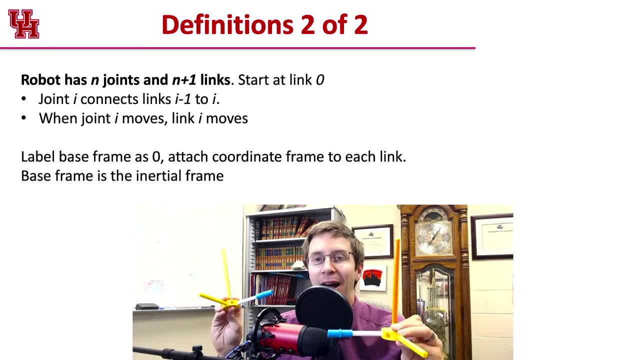 start at link zero and joint. i is going to connect links i minus one to i. When joint i moves, then this link i is going to move, And so we'll label that base frame as zero. We're going to attach a coordinate frame to each link And so the first one is not going to move because that's link zero. 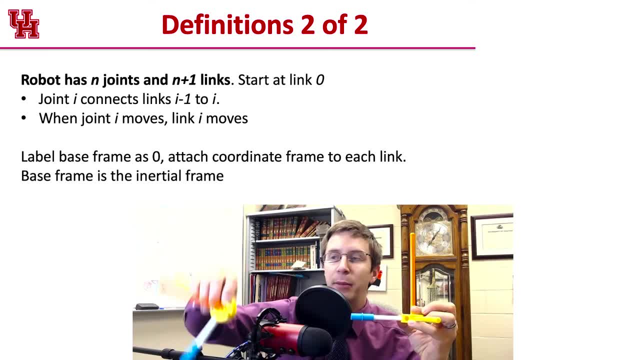 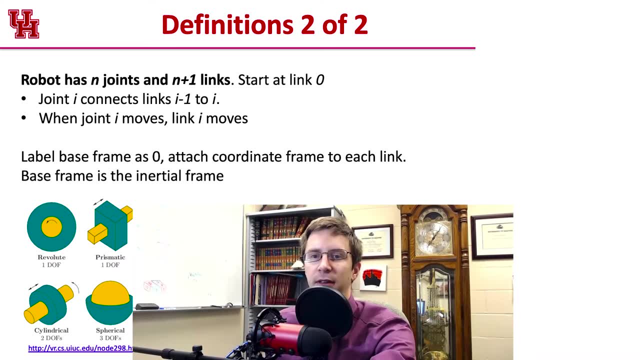 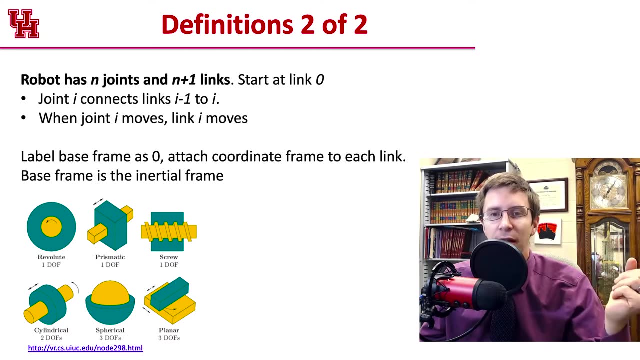 It's our inertial frame, But after everybody after that is going to move. You can go online and you can find a lot of other definitions of different types of joint. In this class we're going to limit ourselves to the first two, the revolute and the prismatic. You can try. 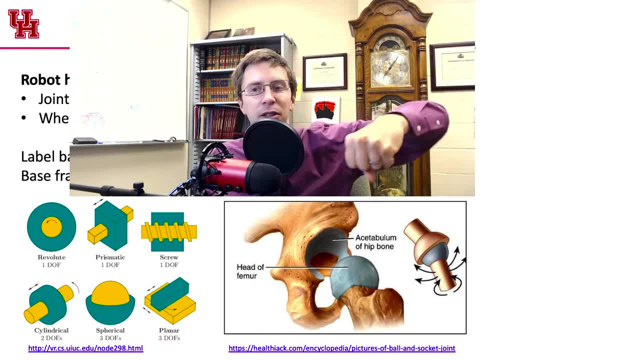 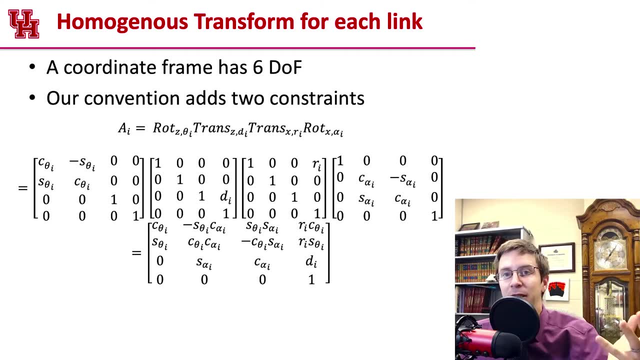 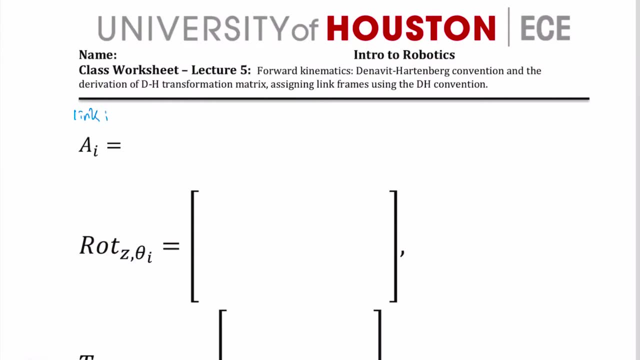 this out with your shoulder, which you can rotate, and you can also pitch in two degrees of freedom. We're going to get started by deriving this matrix, which is AI, the transformation frame for link i. The Navin Hardenberg describes the transformation between link i minus one and 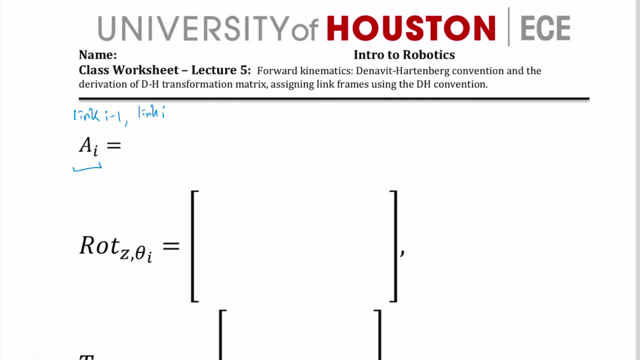 link i, And it does this with a transformation matrix, AI, which is a composition of four different actions. First we have rotation about the current z-axis by theta i. Then we have a translation along the current z-axis by di. Then we have a translation around the current. 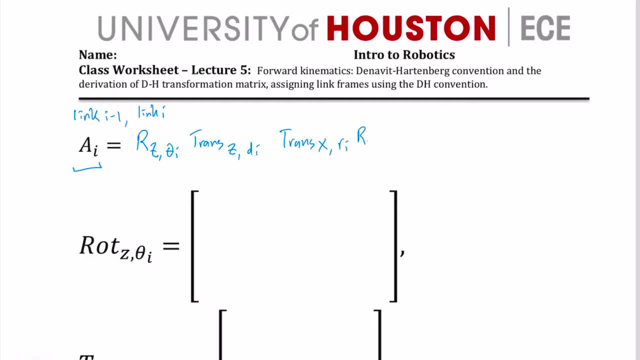 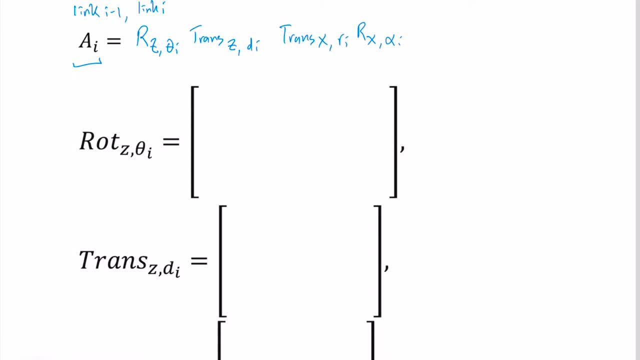 x-axis by ri And finally, we have a rotation about the current x-axis by alpha i. So it's good practice for us to write these out to get practice with homogenous transforms. So, rotation of z about theta i: We're going to have no translation of the origin, or 0, 0,, 0, 0 and our 1 here, And then we 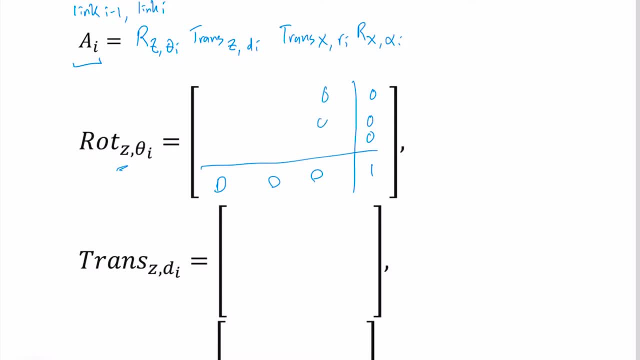 have a rotation about the z-axis So we can put that the z-axis in and then everything that's left rotation. so we get a c theta i negative sine theta i, sine of theta i and a cosine of theta i. then we have a translation along the current z axis. 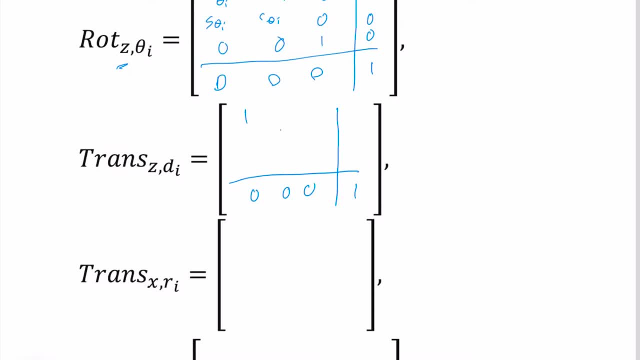 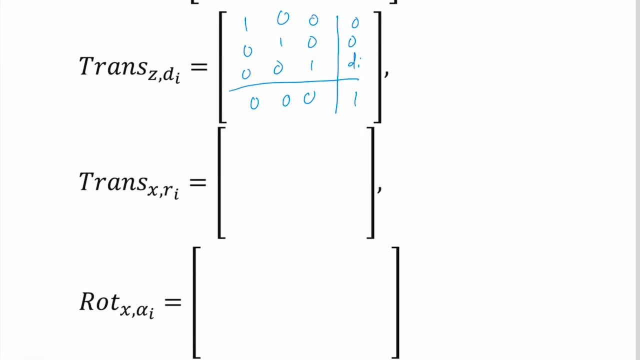 so zero, zero, zero. one is a translation. so we've got an identity matrix for the rotation and then we have everything in the z. so that's zero, zero, d i. next we have a translation along the x. so let's put these guys in again. this time it's along the x. 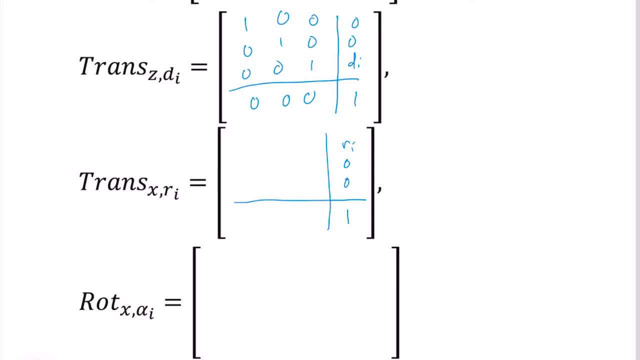 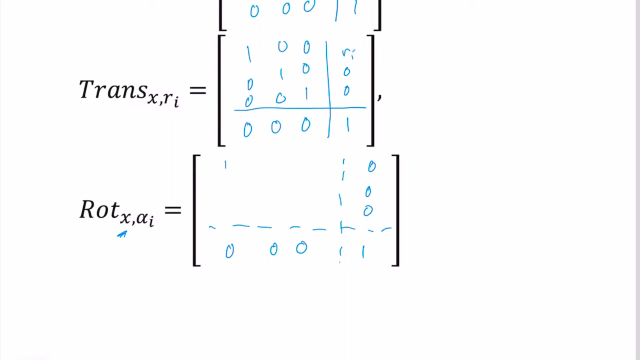 so we'll have r i zero, zero, zero, zero, zero, and then the identity matrix. finally, we have a rotation around the current x axis, so no translation of the origin: zero, zero, zero one here. and we have rotation around the x-axis so we can put a one zero, zero there. cosine of alpha i. 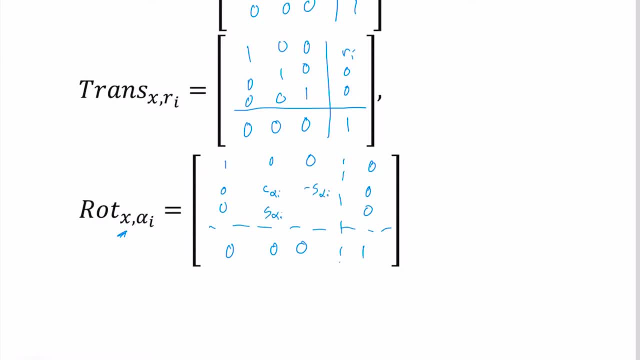 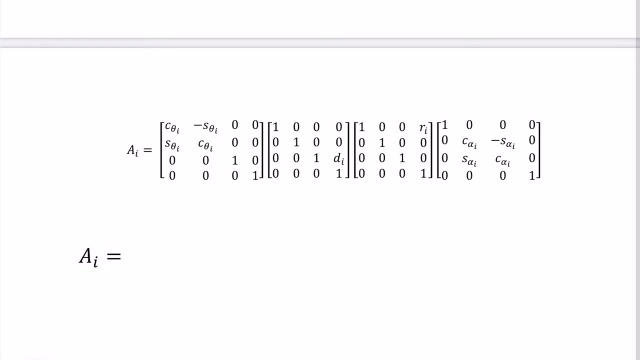 minus, sine of alpha i, sine of alpha i and cosine of alpha i, and there we've got our four translations. so we need to do next is to multiply all these together, and so i've copied these all out and let's just take our time and we'll do that. so i'm going to combine these two together and then these: 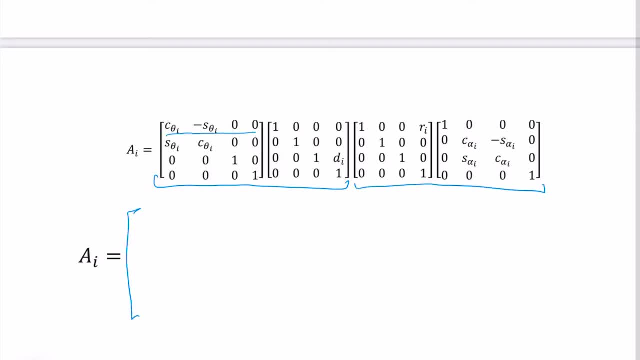 two together. so i take my first row down here. i just get a cosine theta. i take my second row and multiply it across my second matrix. i'll take my first row, multiply it across my second matrix. i'll take my second row and my final row and my final row. 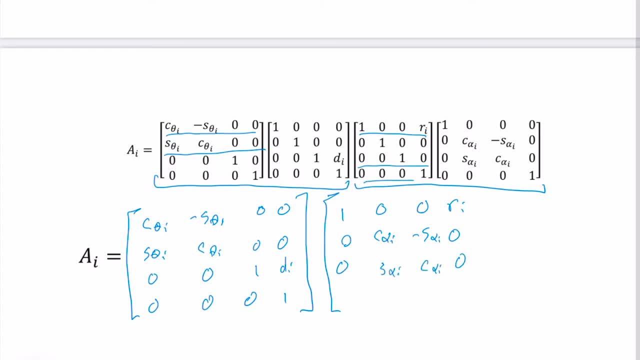 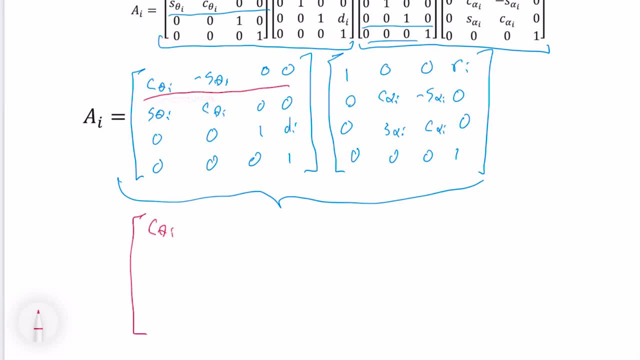 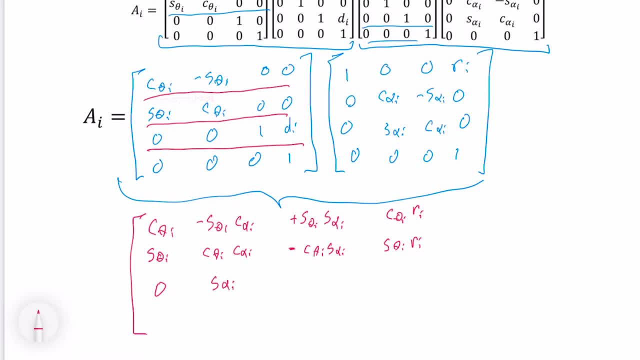 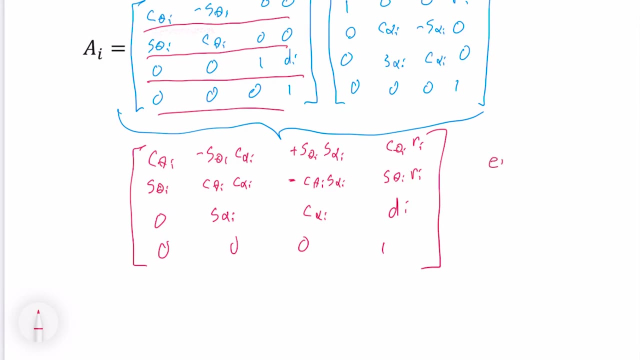 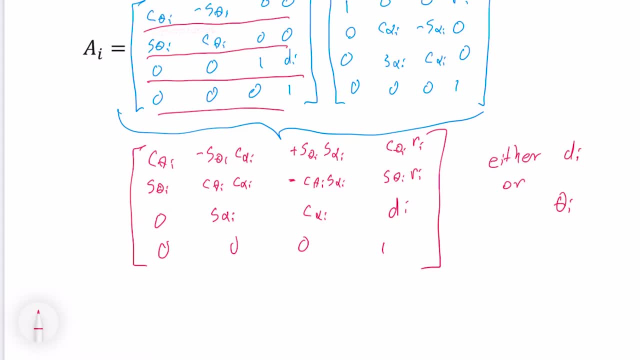 at change. and so we will show which one is the one that changes by putting a star. so it's. and so we will show which one is the one that changes by putting a star. so it's either going to be this or you'll put Perry Bri. 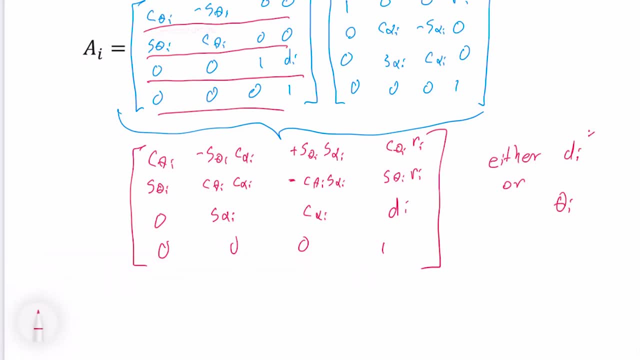 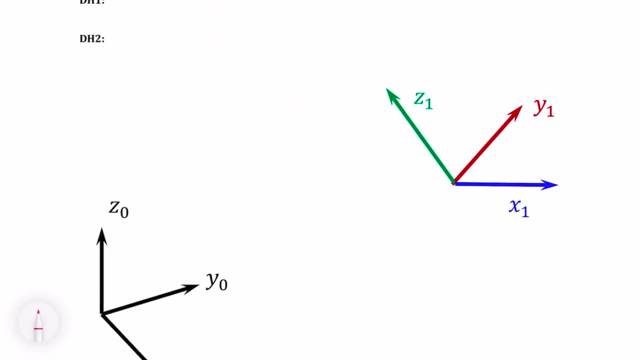 Beckley, a star on the other one, saying that this is a parameter which is not fixed. It is the link parameter that can change. And now it's time for our DH conventions. A rigid body has six degrees of freedom. However, in our Dynavit-Hartenberg, we only have four parameters. 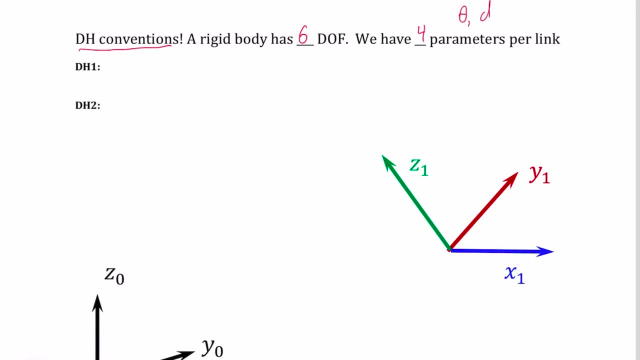 Those parameters again are theta, d, r and alpha. We're going to need some constraints. We need two constraints and that's why we have a DH constraint- number one, and DH number two. The first DH constraint says the axis xi is perpendicular to the axis z0. 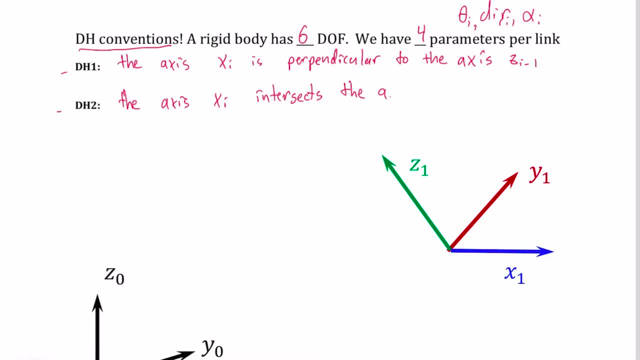 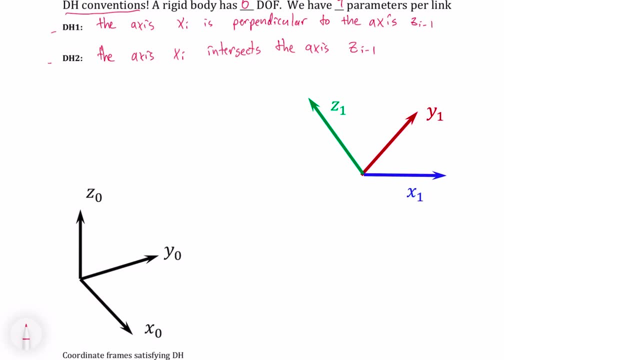 The second DH constraint says the axis x1 intersects the axis z0. And so let's draw out what this looks like. I've got two different coordinate frames, my zeroth and my one, And I want to show how there's this change. 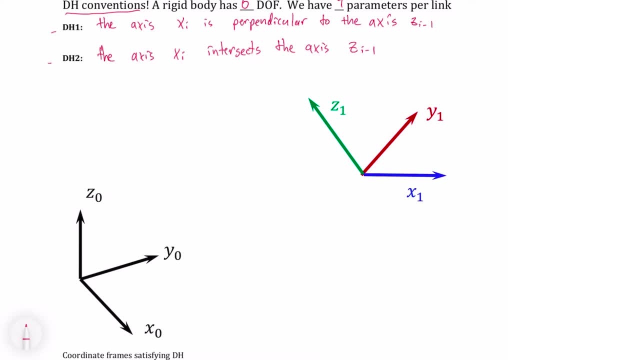 We want to show that there's a change of the origin and of the rotation of coordinate one with respect to the base frame. Our first constraint is that the axis xi, so the axis one, is perpendicular to the axis z0. So we can follow this all the way back here and we can extend this out here. 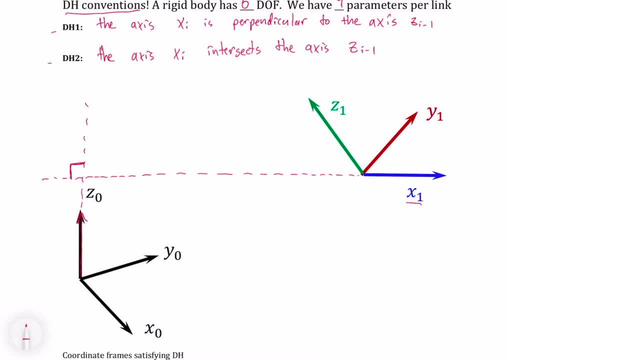 Where they intersect, that's got to be perpendicular. Not only that, but this x-axis also has to intersect, So it's going to be perpendicular to the x-axis. Here, I'm going to take the x-axis. Here, I'm going to take the x-axis. 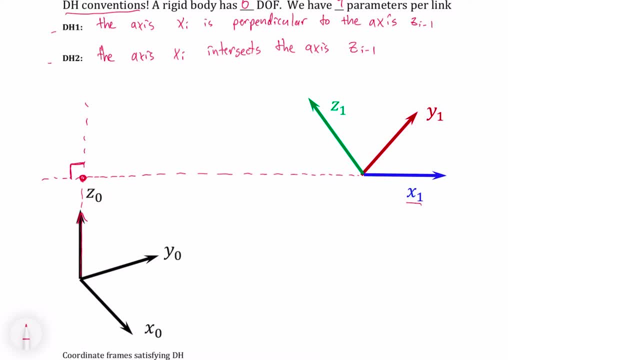 it's going to hit this axis. So let's go ahead and let's draw these on. So I'm going to project this point down into the x0, y0 plane. So I've got right over here. So the first thing we do is a rotation about this z-axis. So we're. 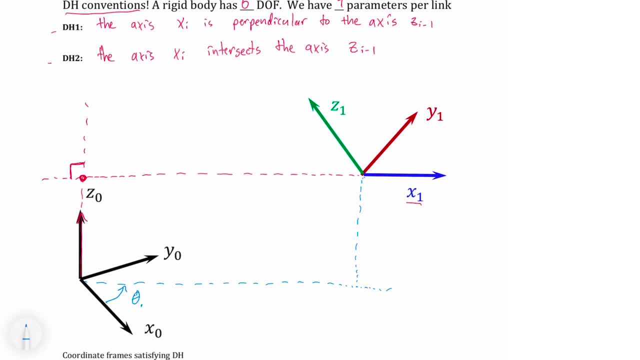 going to rotate over here. that distance that we rotate is theta 1, and then we're going to translate up the z axis from this origin all the way to the intersection point here, and that distance here is dI, And then we have 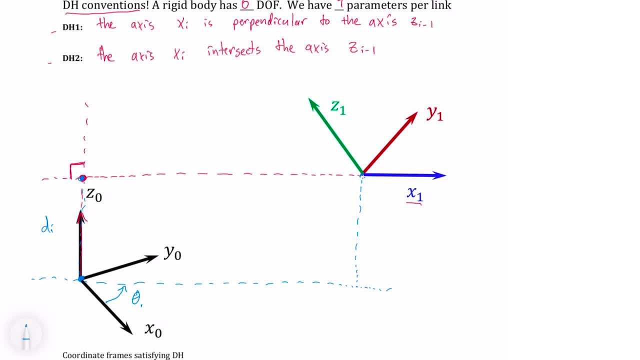 a translation from this point all the way over to the origin of the next frame. that distance is ri. And then we have a rotation about this x-axis little by little in here. So that distance is theta 1, if I cross all my civilizations at this point I will get this senseYer i. And then we have a rotation about this z-axis. 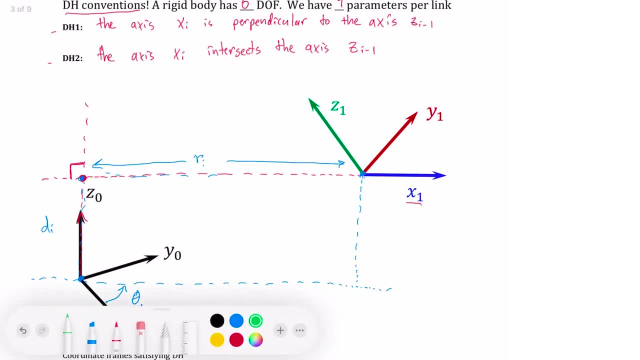 So I'm going to take this z-axis that I have over here and I'm going to put that over here so we can see that This is the translated z0, and that rotation that we do about here is going to be the alpha, alpha i. 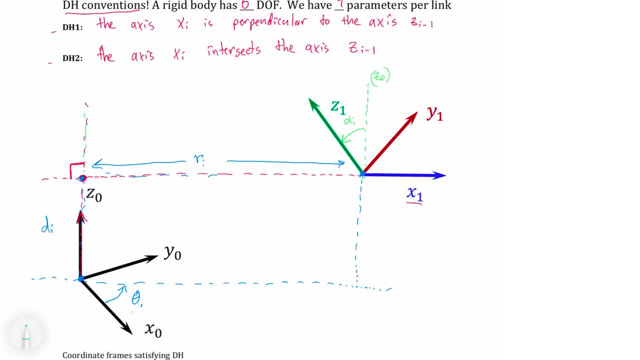 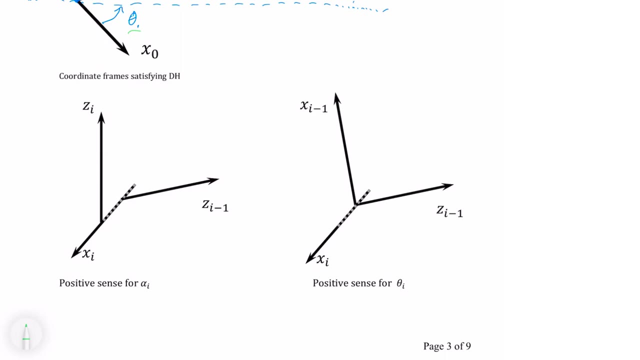 So here we've drawn in our constraints, and so you can see I've got one, two, three, four parameters that describe the origin of this coordinate frame and its orientation. Next, we need to talk about our angle convention for how to describe these angles. 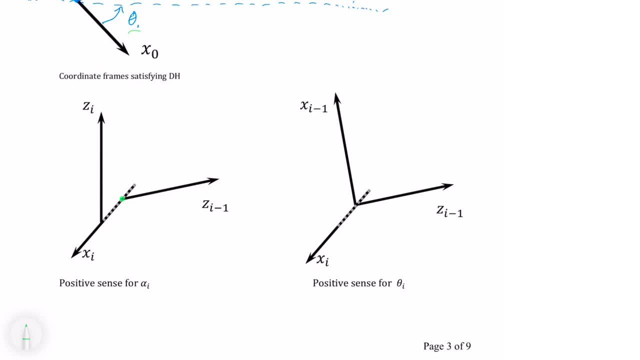 Remember, we've got our previous frame and our x1 intersects that and is also perpendicular to our previous z-axis. So we can translate this z-axis forward to here. So I've just translated that forward and our positive axis is from the previous z0.. 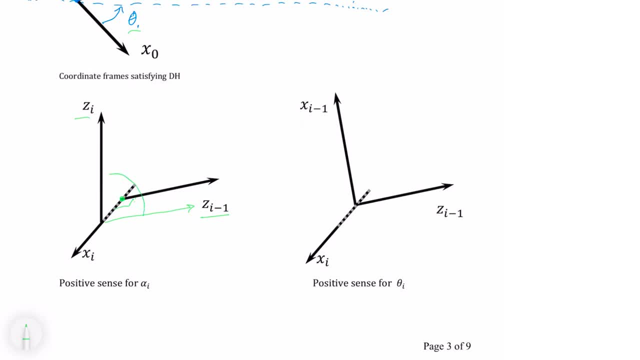 So we're going to go from z to the current z and so we're going to around the current x. So this angle right here, that is alpha i and you can think of that as a right-handed rule. We're going from z i minus 1 to z i about x i. 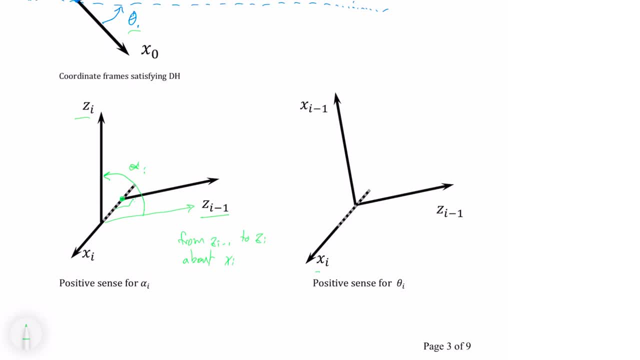 So next one: I've got my x-axis and remember it intersects my z-axis somewhere. But how do I go from my previous x i minus 1 to my current X i? so that rotation that I do there about this axis from here to line up here? that is my theta i. 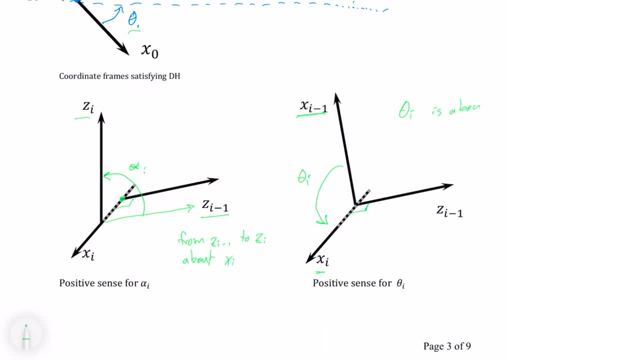 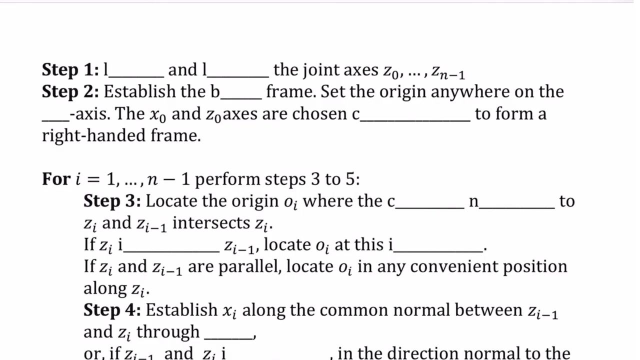 Theta i is about z i minus 1, from x i minus 1 to x i. So I've got this rotation that comes through here. So those are my notations. for which direction is positive rotation? So what the dynamic Hardenberg convention is? it's a series of steps that you can take to establish where your frames are. 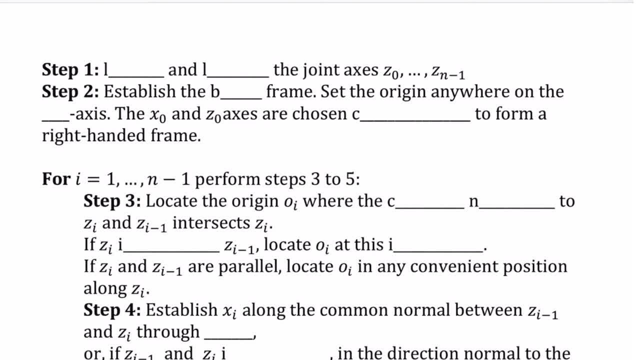 In there. there's going to be nine steps, and let's just walk through them. The first step is we have to tell where the base frame is. So what we're going to do is locate and label the joint axis all the way from z0 up to zn minus 1.. 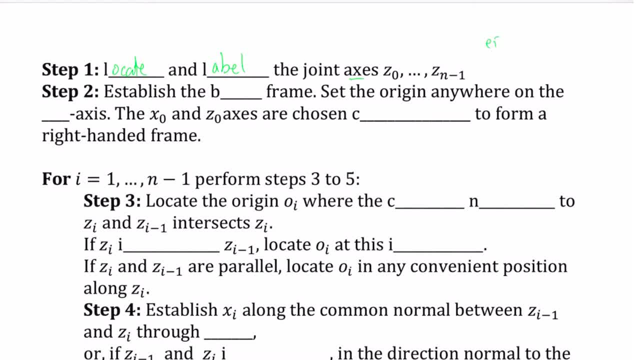 Remember, we know what these are because these are either rotational or prismatic, And so we can just label these joints. where the rotational joints are, We know that the z-axis is going through them, and then we've got a z-axis that's parallel. 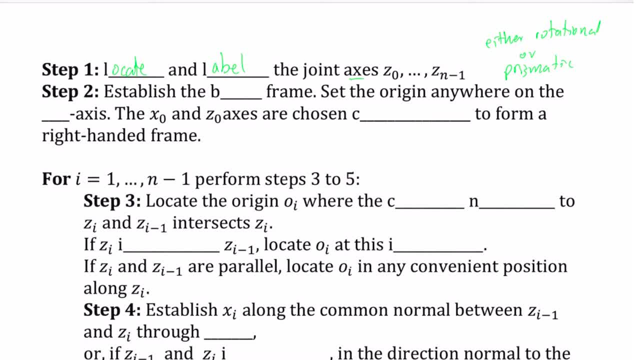 to any prismatic joints. Our second step is we need to establish the base frame, And so we set the origin anywhere. and these are fun things because you can pick your dh parameters to minimize the complexity of the matrix, So you can place that anywhere. 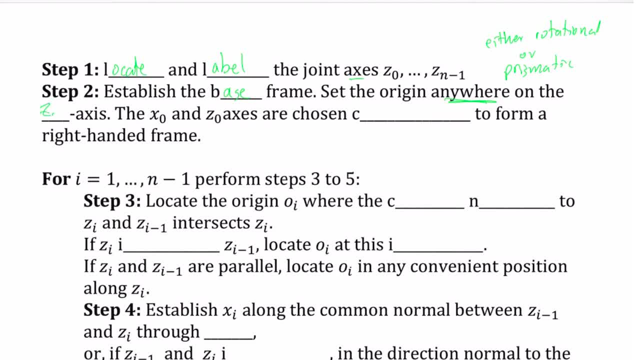 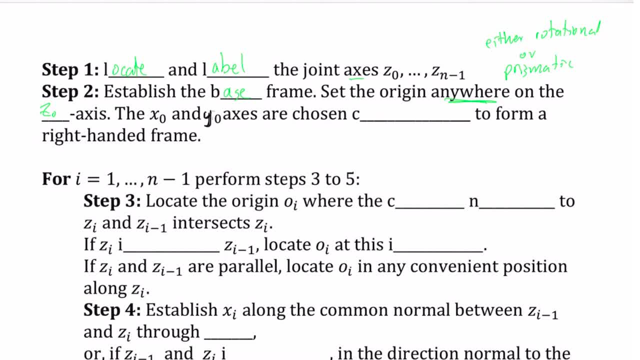 And then we can pick where to place the x0 and the y0 axis. In fact, we can choose them conveniently to form a right-handed frame. So that's the key part: It has to be right-handed frame, but we can put that origin in the direction of x0 wherever we want. 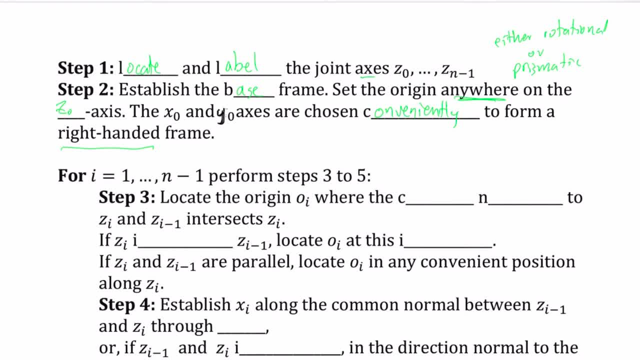 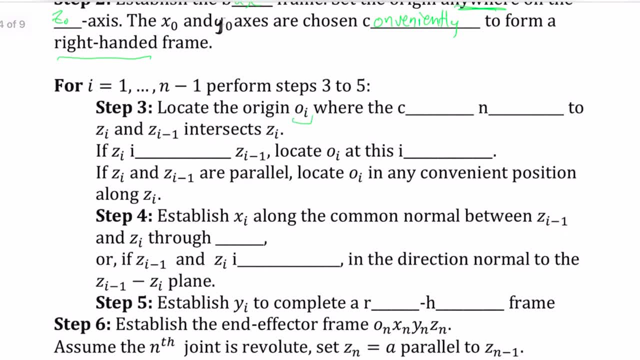 along that z0 axis. And now we get into a loop that we do for every subsequent joint. Step three is to locate the origin oi. And so what we have is we've got our two axes, zi and zi minus 1. We take those two axes, and any time you have two lines, there's always a common normal. 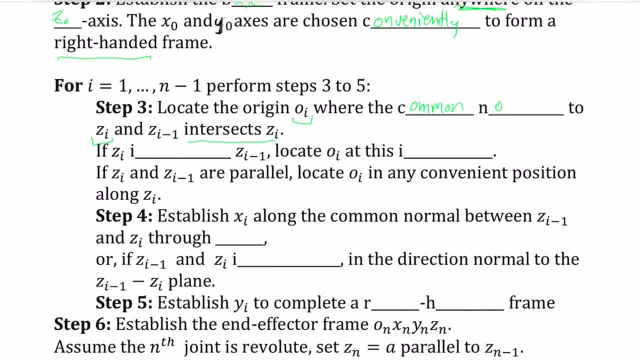 And so we find that common normal, And where that common normal intersects zi, that's our origin. The first one is, if the zi and the zi minus 1 intersect, then their common normal is going to have zero length, And so we're going to locate this oi at that intersection. 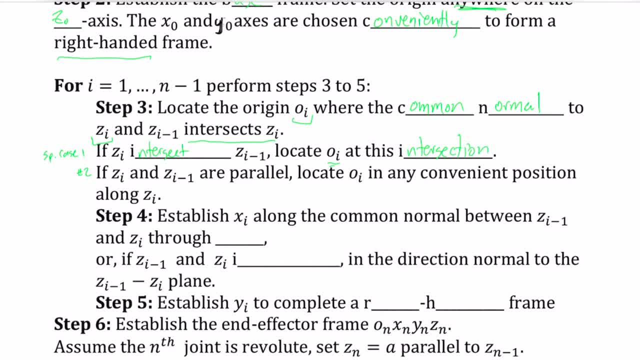 Our other option is if the zi and zi minus 1 intersect. If the zi and zi minus 1 are parallel, then they have an infinite number of common normals. So we're just going to locate it at a convenient position that can minimize the number of dh. 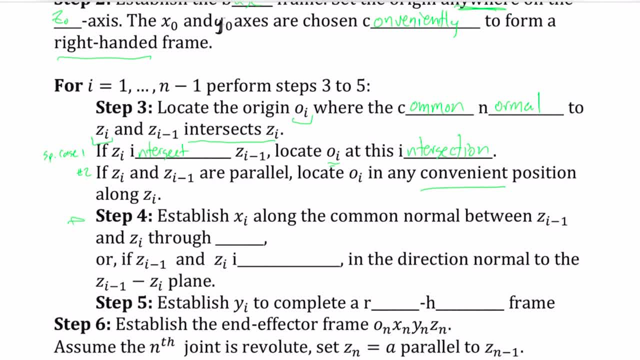 parameters we have. There's some freedom in that one. Our step four: we need to establish which direction xi is. We don't have freedom along that. It's got to be along the common normal between the zi minus 1 and zi and it's got to go. 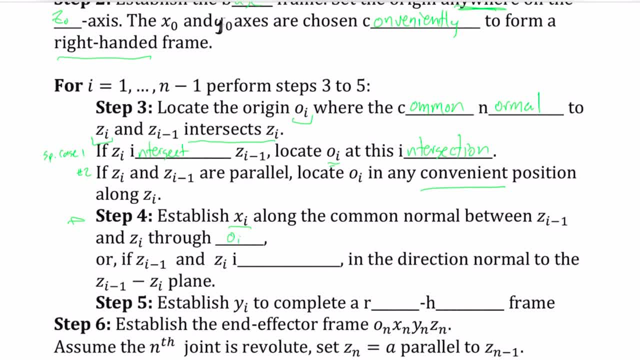 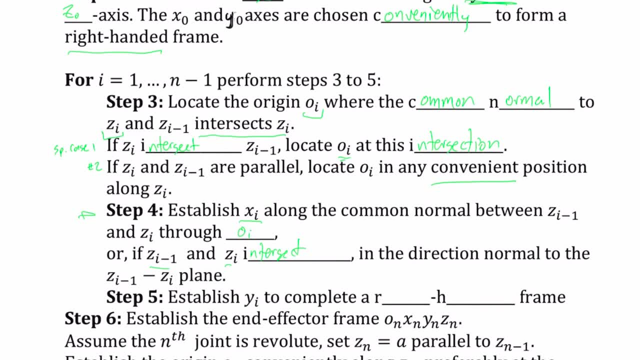 through that origin point that we just described in step three. Now if zi minus 1 and zi intersect, Then we just go in the direction that's normal to the zi minus 1 zi plane. So I can draw that over here. I've got these two x's, zi and zi minus 1.. 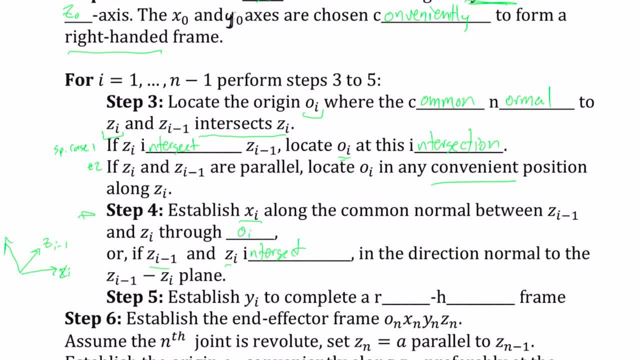 Well then, normal to this frame, we're going to have our x value. Then, finally, step five, we're going to establish where yi is. Again, there's no freedom in here. If you have your origin ori and your xi, then we just need to construct a right hand frame. 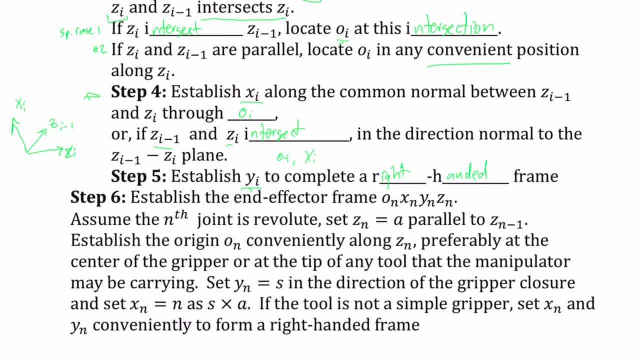 And then step six, we're going to establish where the end effector frame is, And there's two options. If it's a revolute joint, then commonly we set the zn axis parallel to the previous z axis And we put the origin conveniently. 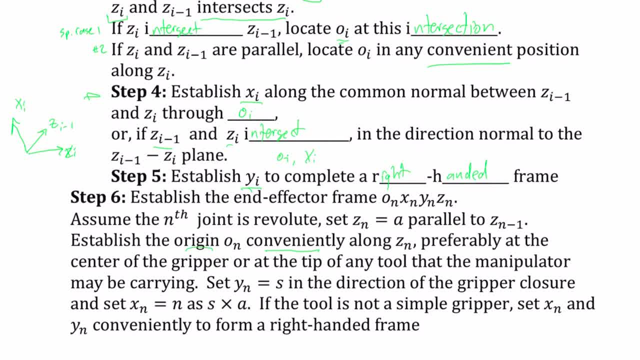 Do you want your origin to be in the middle of your gripper or do you want it along the tip of the gripper? And then we usually set our y direction, the direction of gripper closure, And then our x, And then our y. 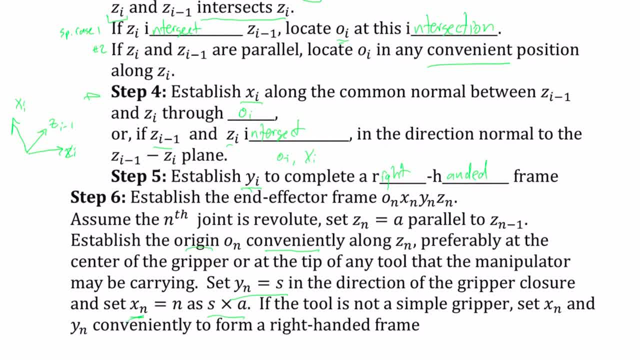 And then our xi is not free because it's just given by the cross product. If it's not a simple gripper, then we can again just set it conveniently to form a right handed frame. Typically what I'll do in the exams is: I will tell you where this last frame is, because 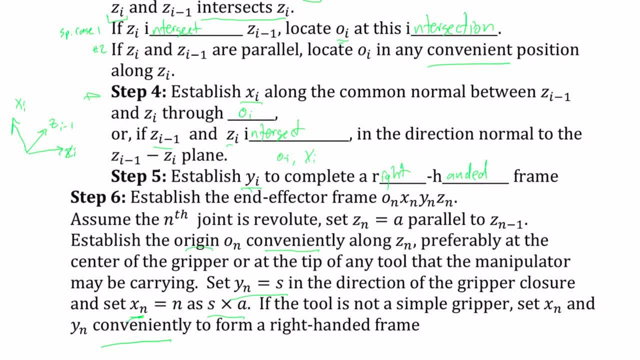 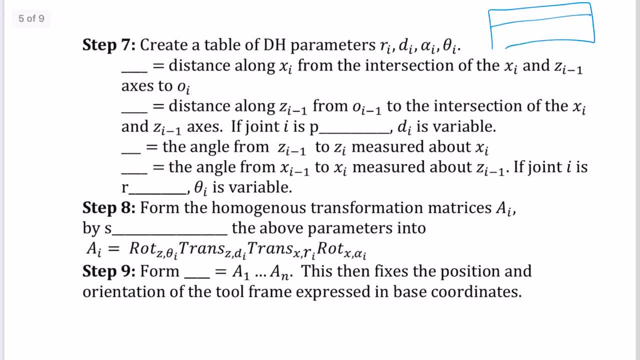 there is some freedom in building this and it's difficult to grade when there's so many options that are possible. Okay, now we're ready for step seven, where we're going to build a table of all the parameters. This first parameter here is the distance along xi. 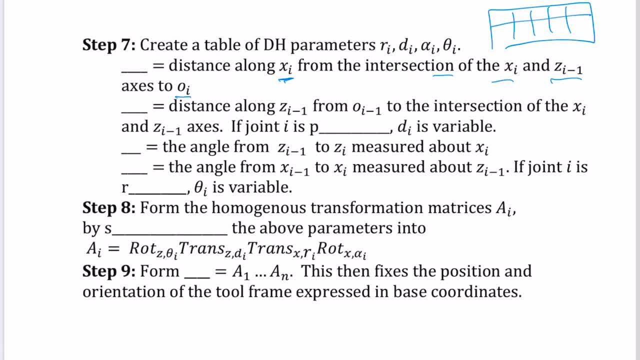 And so this is, from the intersection of the previous axis to the current x axis, My radial distance that I'm rotating. so that's ri. The next one is the distance that I'm translating up along my previous z axis, from my previous origin to the intersection of my xi with this axis. 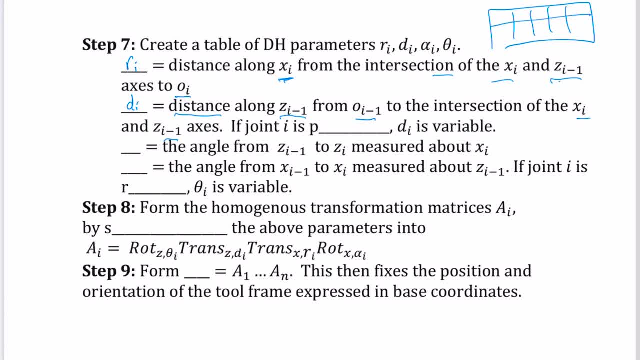 So this is my di, how much I translate up that z axis. If that joint i is prismatic, then d is variable. Okay, Okay, So we'd write di star, showing that it's variable. Next, I have the angle from zi minus one to zi, measured about my x axis.